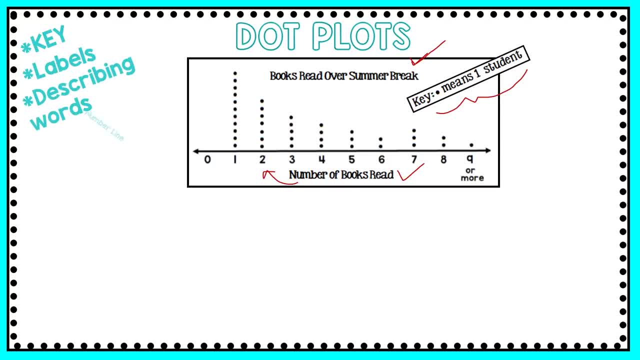 that's telling me that these numbers represent the number of books. read The describing words. pay attention to those. and number lines. Dot plots have number lines. That's a big part of reading a dot plot. So in this case the number line here starts at zero and it goes to nine or 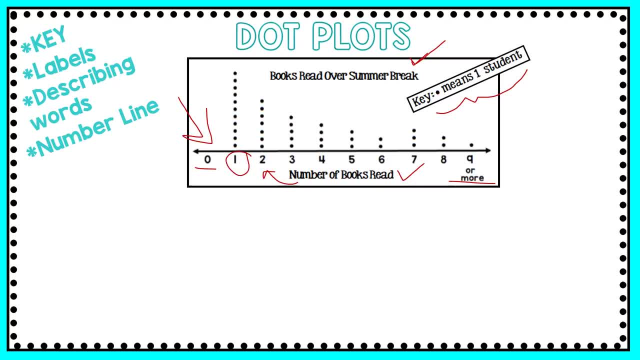 more. So if I'm looking to see how many students read one book over the summer, I will look at this column. So when I count the dots, I know that 11 students read one book over the summer. Now it's important to know on dot plots if you don't have a key, if there's no key on the dot plot, then you're safe. 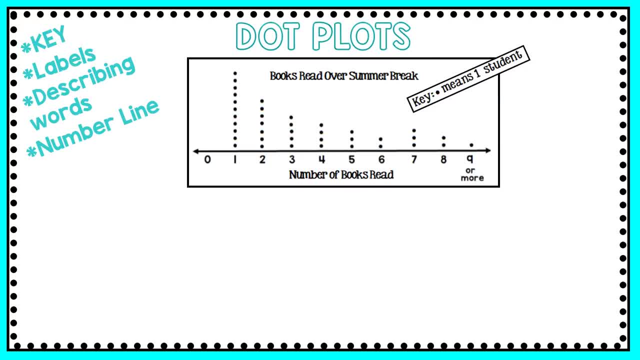 in assuming that every dot means one. Let's take a look at another dot plot. Here's one where you don't necessarily have dots but you have circles. and let's look at those labels and describing words. I see number of pets is my title. number of pets at home. 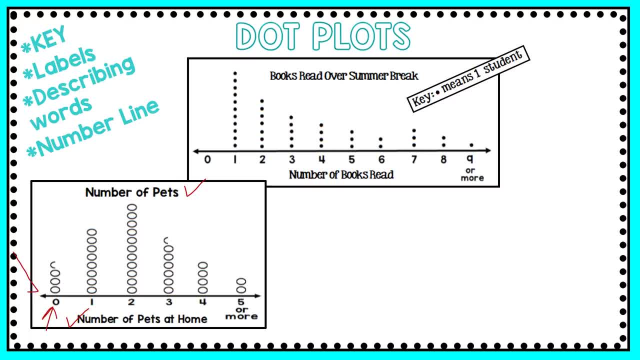 are the numbers below. Here's my number line, and so let me see what my key tells me. The key is telling me that every time I see a circle, that represents four students. So when I'm looking at this dot plot, I'll count each of these symbols by four. Let's look at another dot plot, On this one. 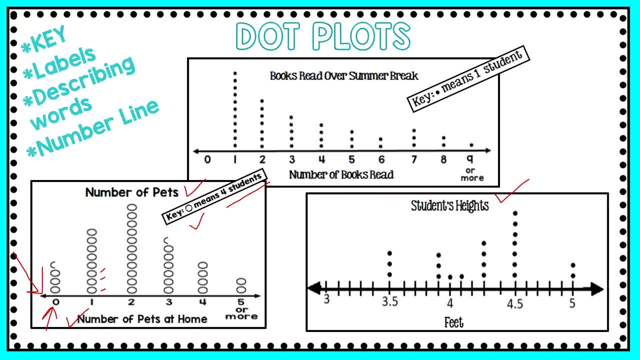 you see that your dot plot is about student heights. The heights are measured in feet and you have decimals on this dot plot. You're going to be reading a dot plot and you're going to be reading dot plots with decimals. You'll see that this number line starts at three and it goes up to: 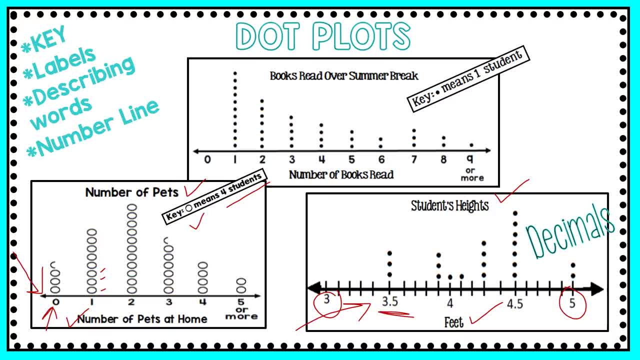 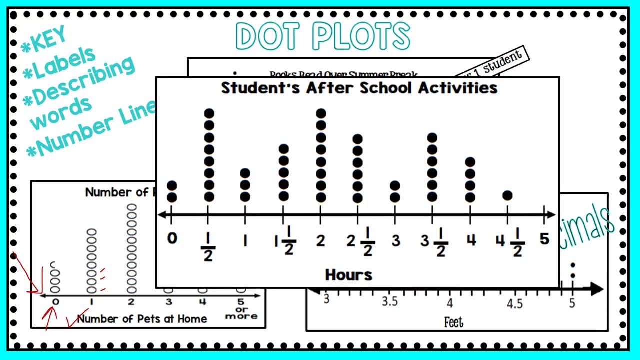 five, and so you see the number of students who were three and five tenths feet tall were three. Let's look at one more dot plot on this slide, and this one is also read using fractions. You're going to be reading dot plots that include fractions, and this one you can see is counting. 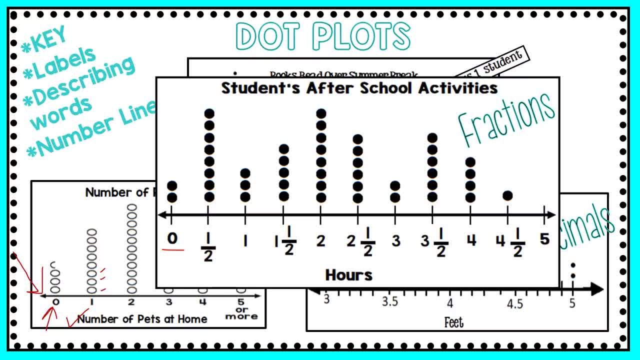 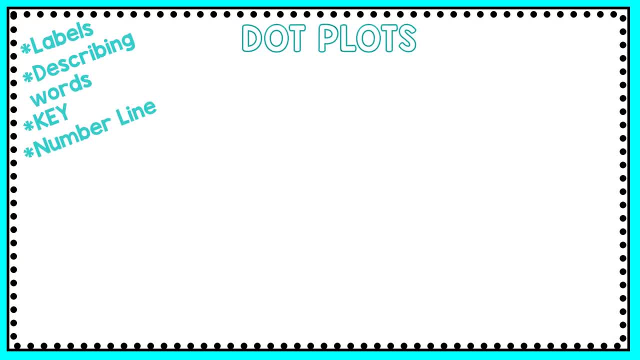 by halves. So it's going to be reading by fractions. You're going to be reading by fractions: Starts at zero and it ends at five, and each increment is counting by halves. Let's look at a few more examples and remember to keep these things in mind whenever you're looking. 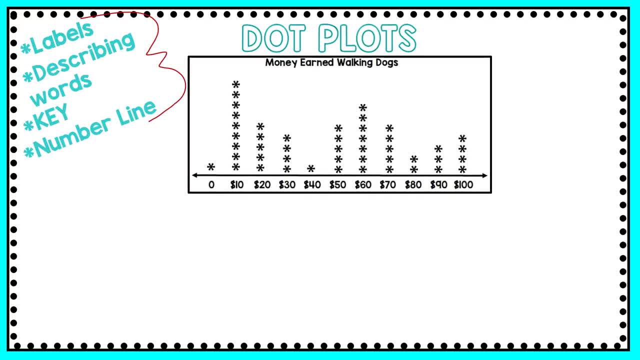 at dot plots or graphs. Here is a dot plot where it's not dots at all but it has stars or symbols and you see your number line and you have money represented counting by tens at the bottom On this dot plot. you see that you don't count byosium numbers. you see a dot and a dot and a dot. 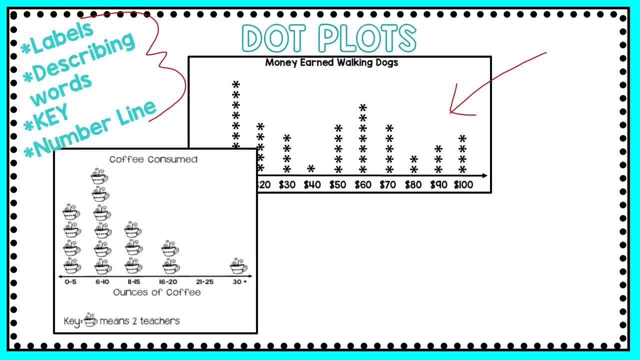 you don't have dots at all, but you actually have pictures, and this one is about coffee consumed and you have pictures of coffee cups and here's your number line and the range. so the number of ounces consumed by teachers are 0 to 5 and 6 to 10. so that's how that number line is counting. another example of a 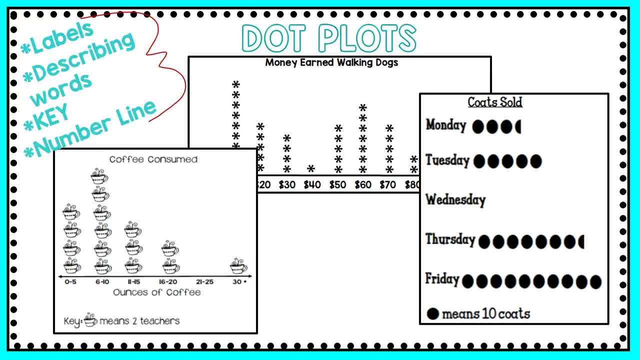 dot plot that you may see is this one. now, this one stands out because the dots are not moving bottom to top or vertically. they're moving left to right or horizontally. so you'll often see dot plots where the dots are moving bottom to top, but you won't always see those. in this case, this one has the dots moving. 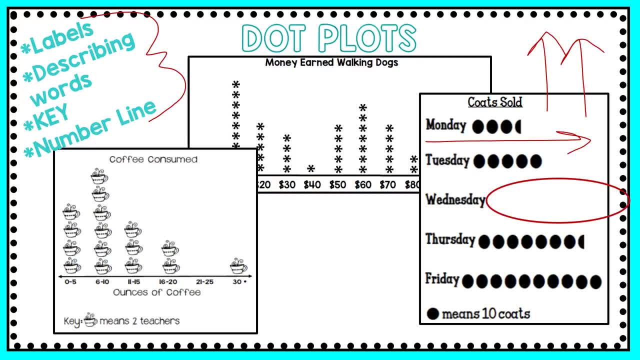 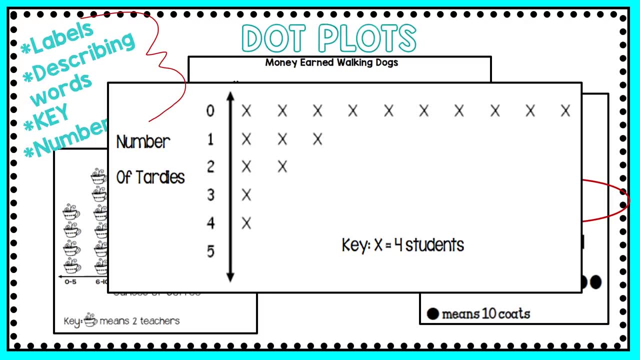 left to right, and it's also missing some information. you're missing information on this dot plot, so you may encounter some of those. and then one more example of dot plots that I'd like for you to see is this one. it's similar to the one I just mentioned. as you can see, your dots are X's and you have a number. 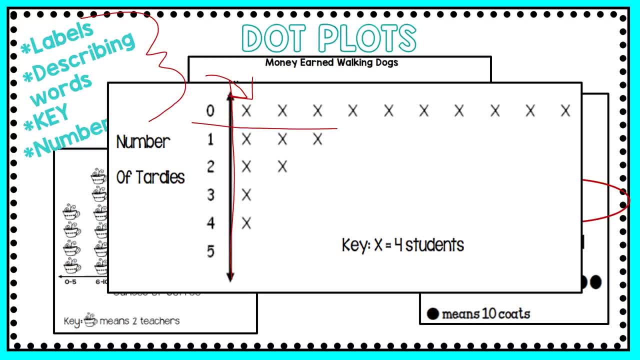 line moving up and down, and zero is moving across this way. so this is about tardies, and my key tells me that every X represents four students. so the number of students with zero tardies are in this row right here. so these are just some examples of dot plots you might encounter. so let's answer some questions. 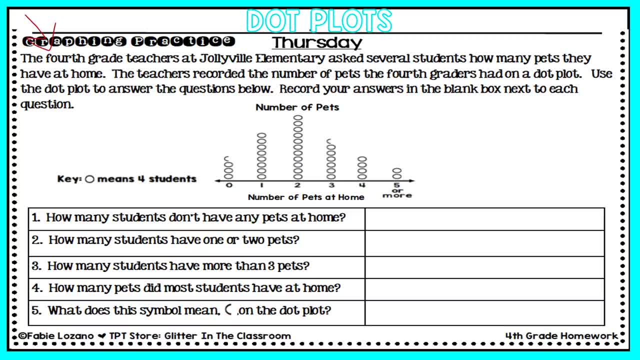 first here. so a half grade teachers at Jollyville Elementary asked several students how many pets they have at home. the teachers recorded the number of pets the fourth graders had on a dot plot. use the dot plot to answer the questions below. record your answers in the blank box next to each question. so let's take. 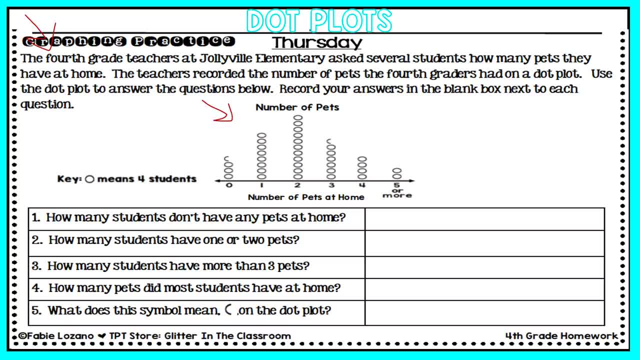 a look at our graph now. remember to pay attention to those labels and descriptors. the title is the number of pets. my labels at the bottom tell me number of pets at home and that means at home one is one pet. at home two is two pets, and so on. Now remember I told 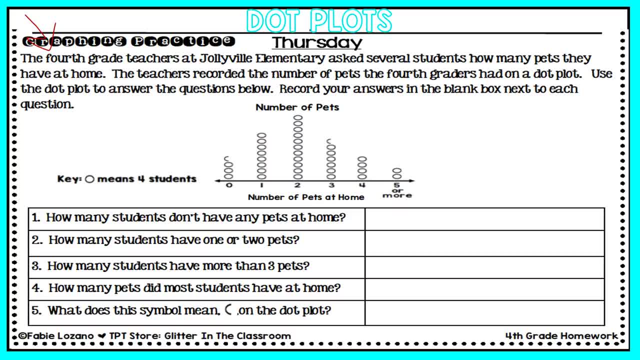 you to pay close attention to that key. I tell my students to make the key stand out. If we don't have the key correctly, then we won't answer the questions correctly on the graph. So the key tells me that every time I see a circle it 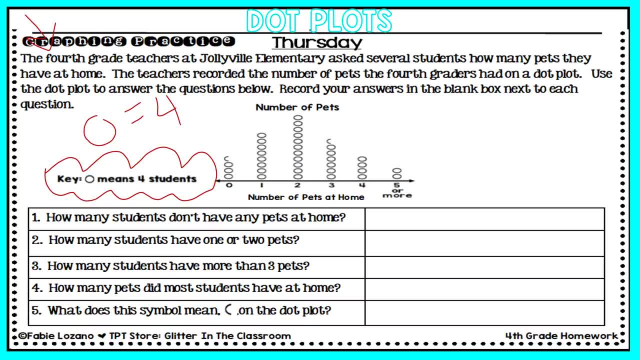 represents four students. So let's label this graph before we even get started with these questions. Now, this graph has circles that represent four. So the number of students who have zero pets is four, eight twelve, and I see a half of a circle. So if one whole circle equals four students, then a 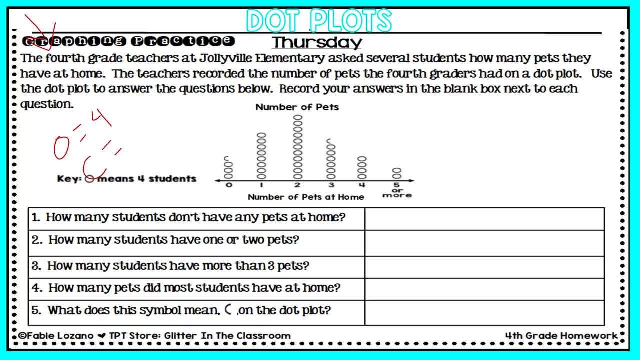 half a circle must equal: half of four is two. so the number of students with zero pets is four, eight, twelve, three, four or two, and then I'm going to add that to That's 14.. The number of students with one pet at home: If I count those, I'll see it's. 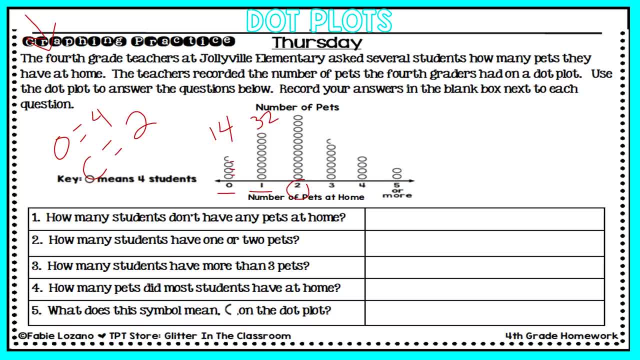 32.. The number of students with two pets at home- This looks like my highest number- is 44.. The number of students with three pets at home is 26.. Four pets at home is 16, as I count those, and five or more. 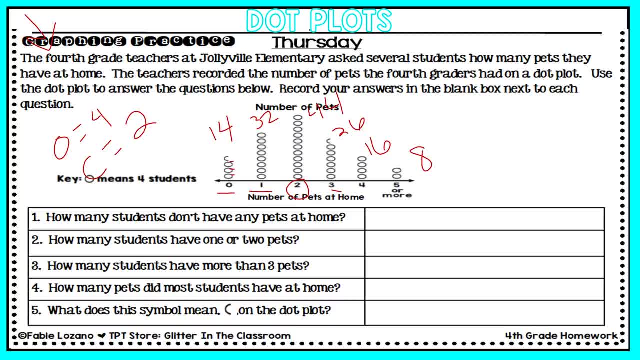 pets at home. How exciting, that's: eight students. So now I'm ready to answer my questions. Number one: how many students don't have any pets at home? That means zero pets, and I know that was 14 students have no pets at home. Number two: 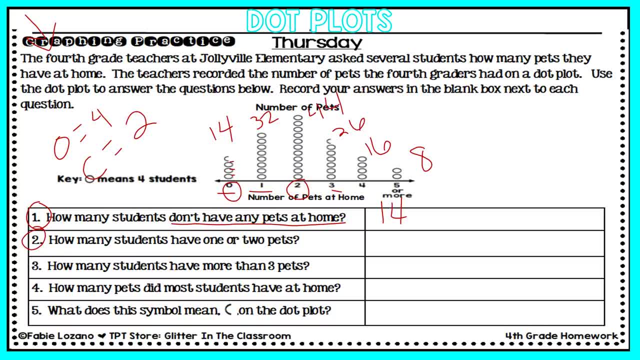 how many students have one or two pets. So on questions like this, you have to look at more than one piece of data. One pet was Here and that's 32 students. Two pets was here and that was 44 students. so I have to take 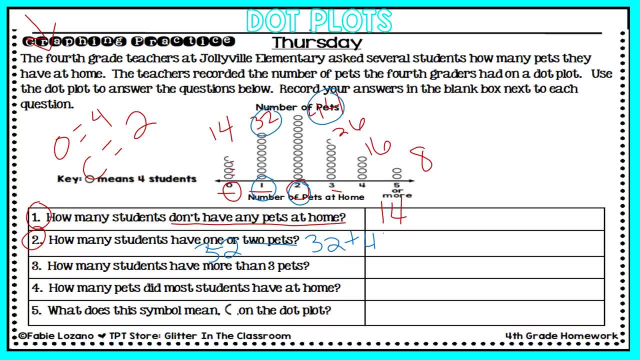 32.. Plus 44 because it represents one or two pets, and I'll let you do that on your own. That's gonna Give me my sum, and my sum is what I'm looking for here. So let's go to number three. How many students have more than?